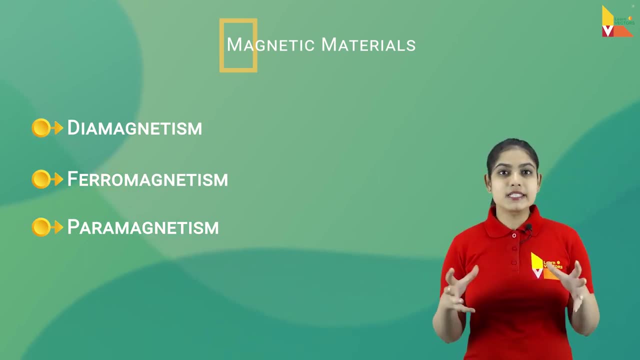 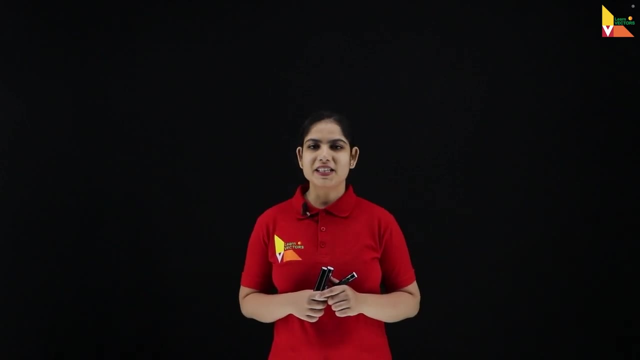 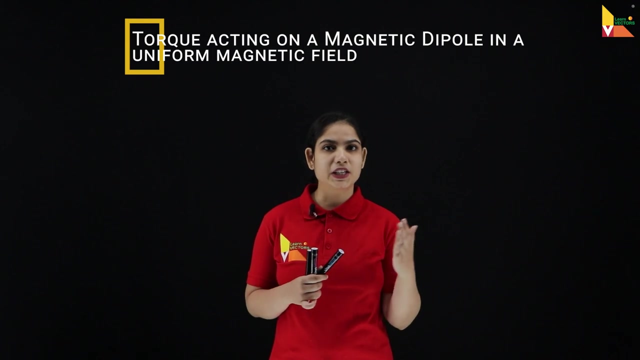 of the magnetic materials. So this is all that we are going to study in this chapter. So let us start with the first topic of this chapter. The topic is the torque acting on a magnetic dipole in a uniform magnetic field. Now, whenever we are discussing about a magnetic field, 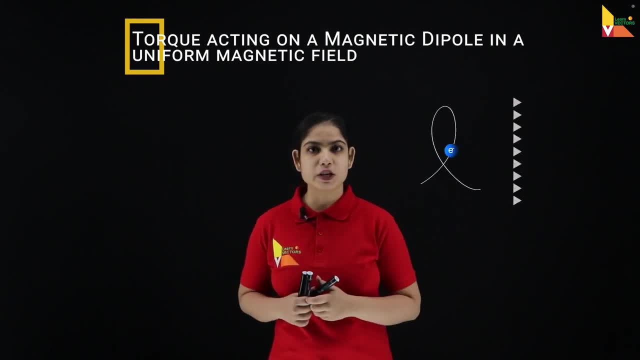 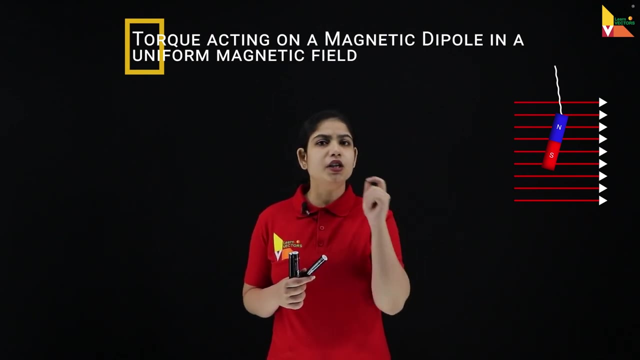 we have studied that electric current generates magnetic field around it right. And if in this magnetic field suppose we suspend a bar magnet, then we observe that the magnet is deflecting right. So a torque is acting on that bar magnet right, And the torque because 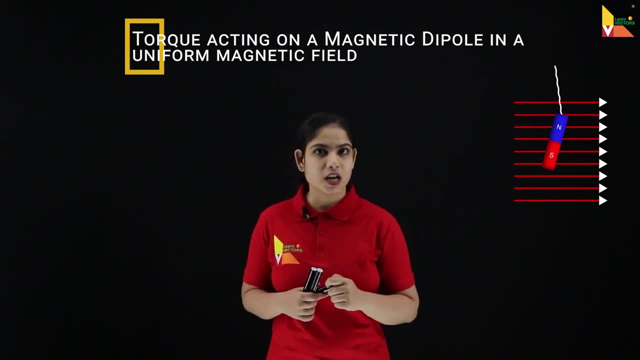 of the torque. there is a displacement in this bar magnet right, And displacement results in what Change in potential energy? right, We have also learned about this that whenever an object is being displaced, some work is done on that object, right? Whenever the object is being displaced. 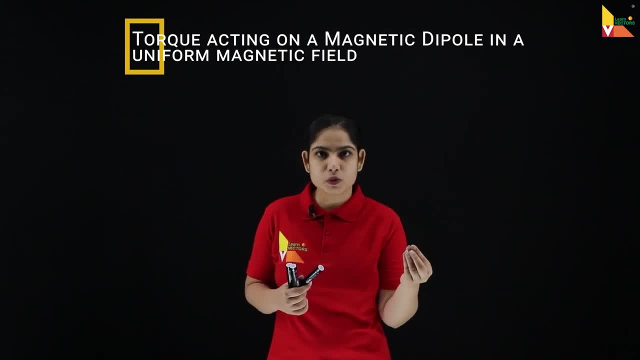 at that time, some work is done on that object, and this work done is what? This is equal to the change in the potential energy right, And in this topic, this topic is basically divided into three portions. The first portion is about the torque of the bar magnet and the second portion 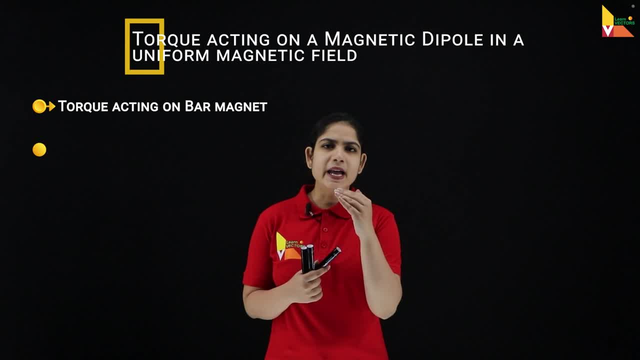 is the potential energy right. So we can relate these two portions, the first part and the second part. Because there is a torque, there is displacement. Because there is displacement, there is work done, and because there is work done, there is a potential energy, change in potential energy. 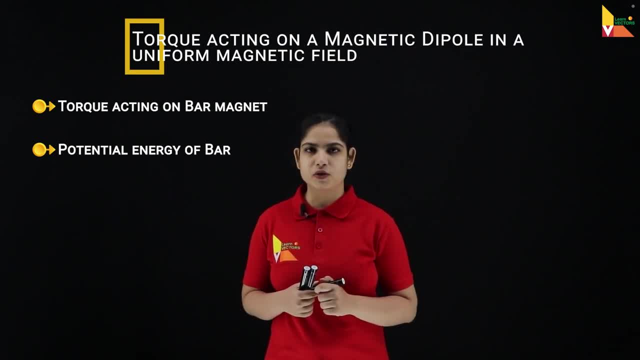 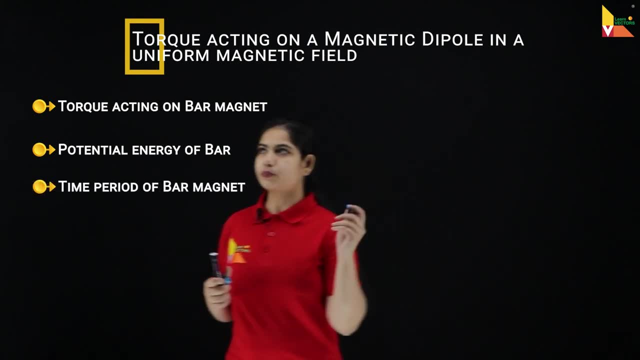 right, And we have to find out this change in potential energy. and the third section of this topic is what To find out? the time period of the bar magnet. okay, So this topic is basically divided into three parts. In the first part, we are going to talk about the torque of the bar. 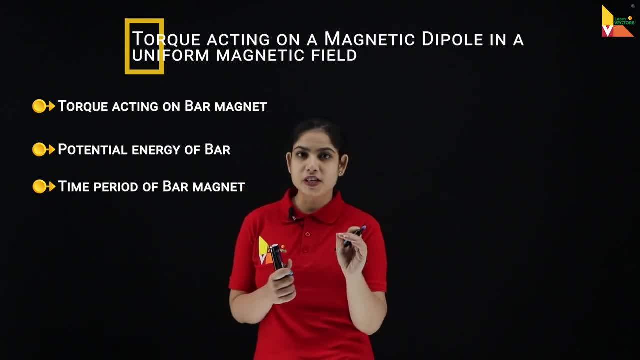 magnet. In the second part we are going to talk about what The torque of the bar magnet and the potential energy of the bar magnet, and in the third part we are going to talk about the time period of bar magnet. So now suppose a magnetic field is generated. right, There is a magnetic. 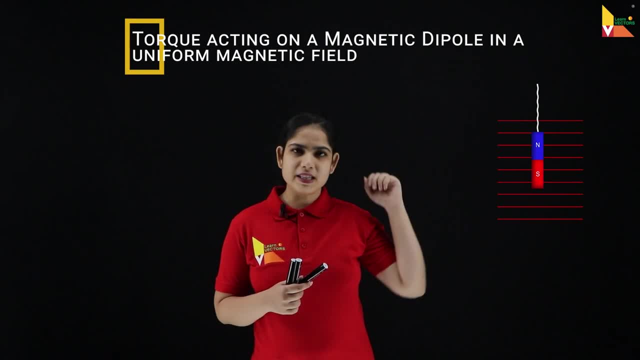 field and a bar magnet is suspended in that magnetic field. Now what will be the direction of deflection? Suppose that we don't know what is the direction of the magnetic field, Then how to find out the direction of the magnetic field? Well, we are going to talk about the direction of the. 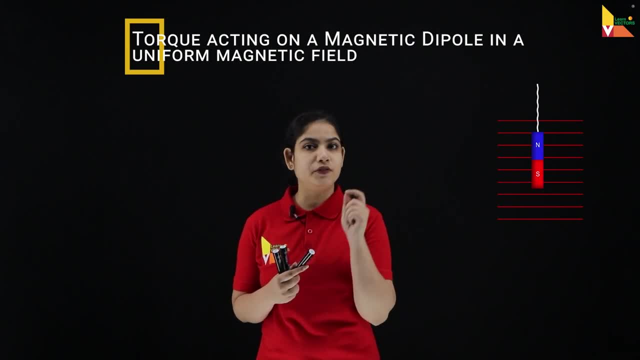 magnetic field. The direction of magnetic field can be found out by suspending a bar magnet in that magnetic field. and wherever is the direction of the north pole? okay, The direction of deflection of the north pole gives us the direction of magnetic field. okay, Remember this That whenever. 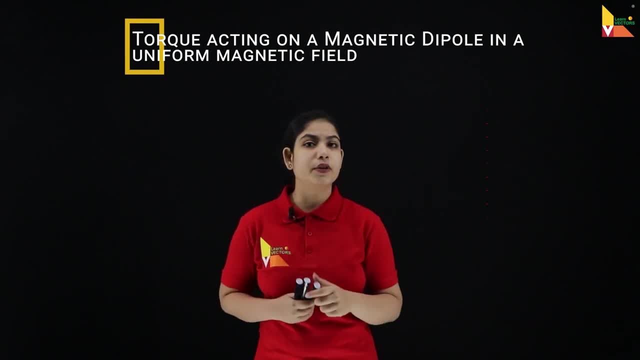 we need to find out the direction of the magnetic field. then what do we do? We suspend a bar magnet in that magnetic field and the deflection, the direction of deflection of the north pole gives us the direction of magnetic field right Now. because of this, first of all, 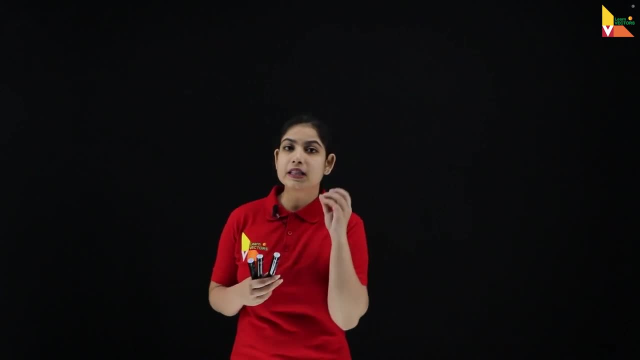 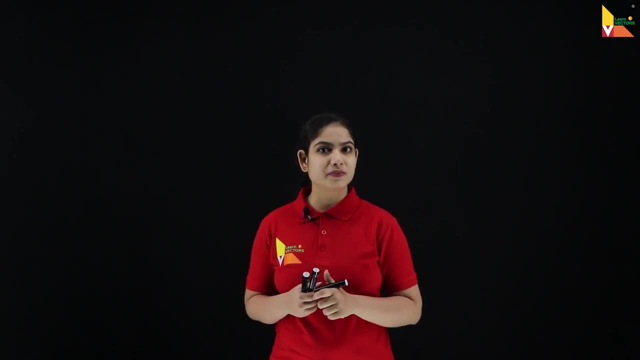 tell me what is the formula for magnetic field? okay, And in this case we are talking about a uniform magnetic field. So what do you mean by a uniform magnetic field? In uniform magnetic field, the magnetic lines are Parallel to each other, right, And they are equidistant as well. So we are considering what A uniform magnetic field. What is the formula for magnetic field? Magnetic field is given by. magnetic field is equals to force upon pole strength. Right, This is the formula for magnetic field. that is what B is equals to F upon MP, Where MP is. 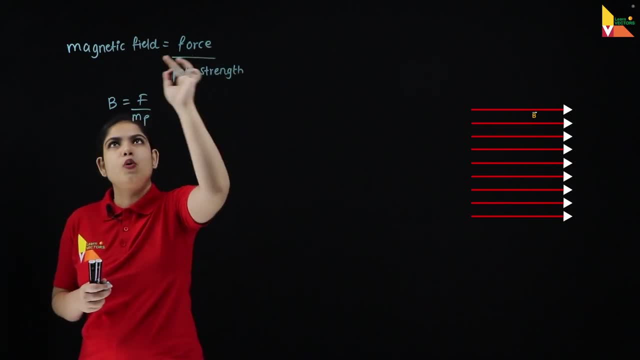 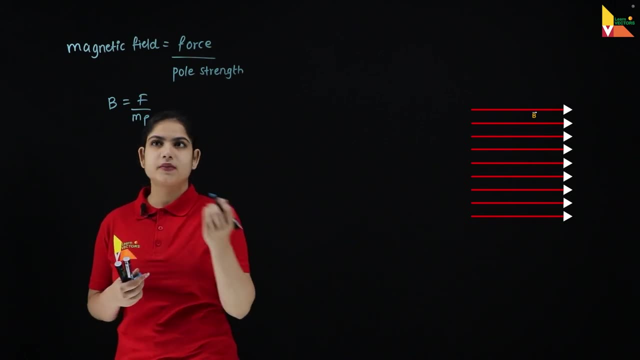 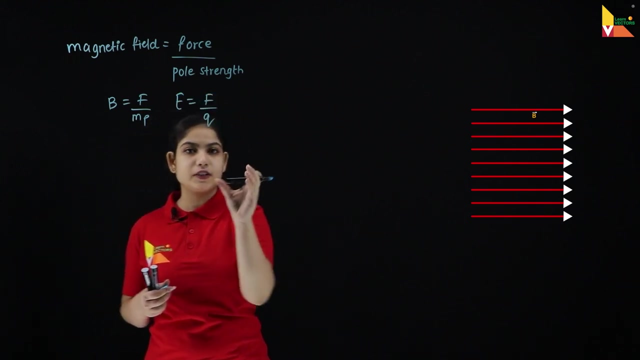 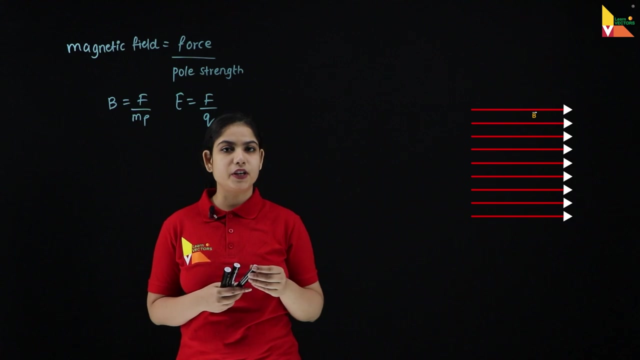 what MP is the pole strength, F is the force And B is the magnetic field. And what is the formula for electric field? Electric field is force per unit charge. right? This magnetic field and electric field are each other. that is why we study about both these simultaneously, but in this part we are. 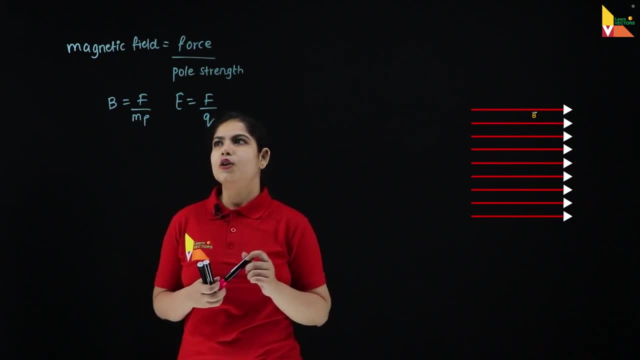 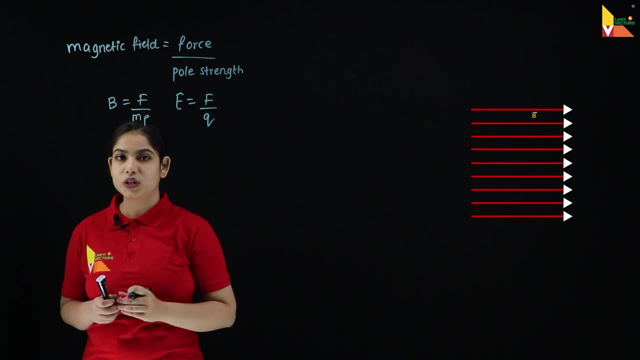 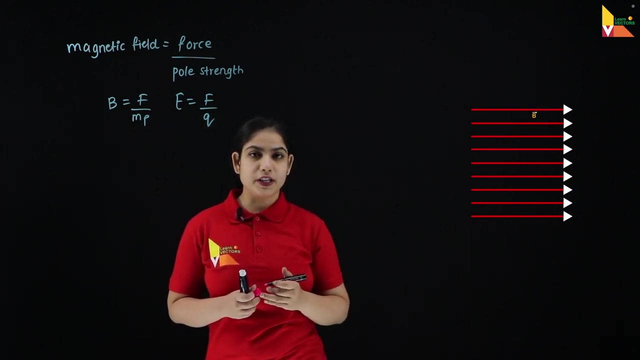 going to study about the magnetic field only, right. so over here, the magnetic field is what it is, nothing but the ratio of force and pole strength. MP is the pole strength, okay, so now, if we look at this figure over here, because of the magnetic field, the bar, magnet experiences. 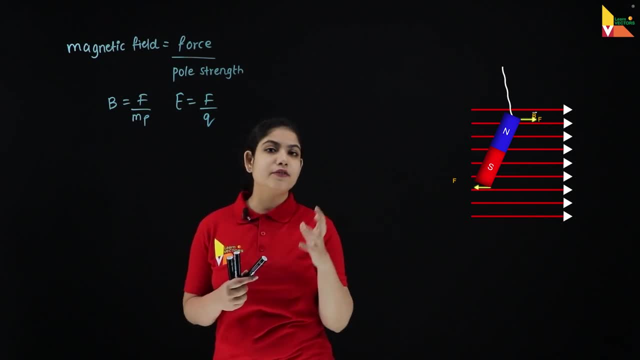 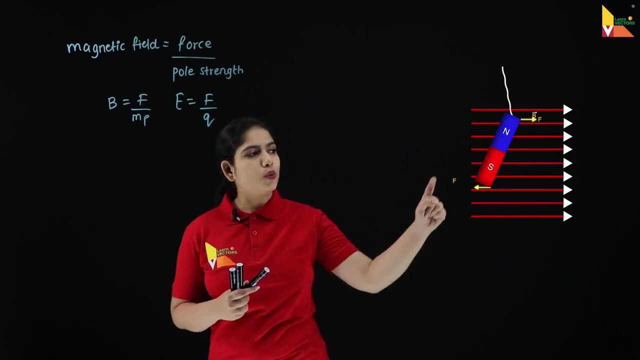 torque right, and because of this torque, there is a force experienced by both the poles, the North Pole as well as the South Pole right. so now, what will be the direction of force of the North Pole? the direction of force of the North Pole is along the direction of the. 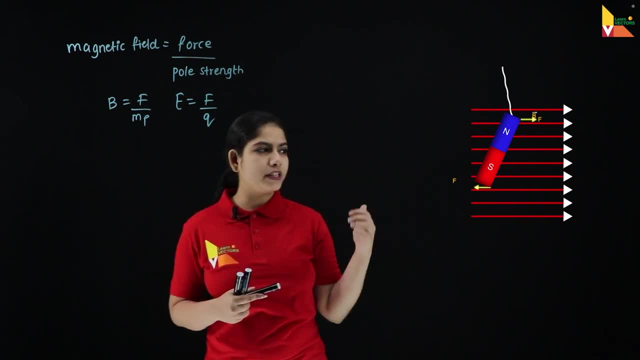 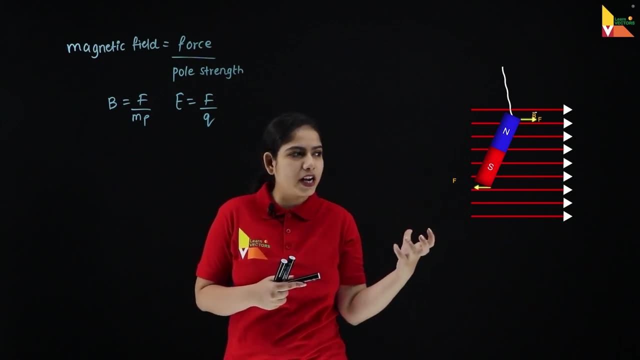 magnetic field. right, in this case we know the direction of magnetic field and by using the direction of magnetic field we are trying to find out the direction of magnetic field, North Pole, the direction of force experienced by the North Pole. okay, but suppose, if we do not know the direction of magnetic field at that time we are going to suspend that bar magnet and 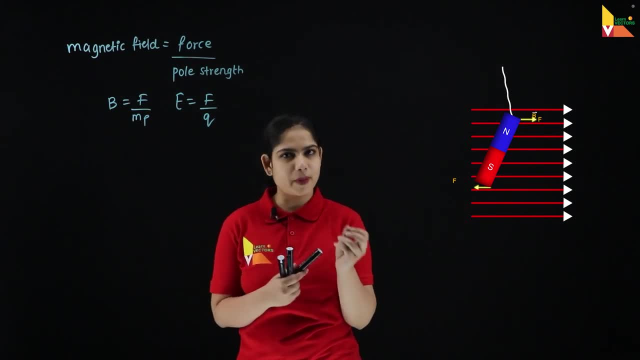 likewise, we are going to find out the direction of magnetic field. according to what? according to the direction of deflection of North Pole, right, so over here, the magnetic field is given and in this magnetic field we are suspending a bar magnet which is experiencing torque. and because, 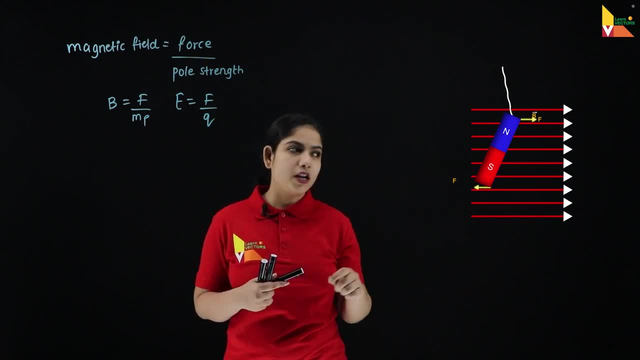 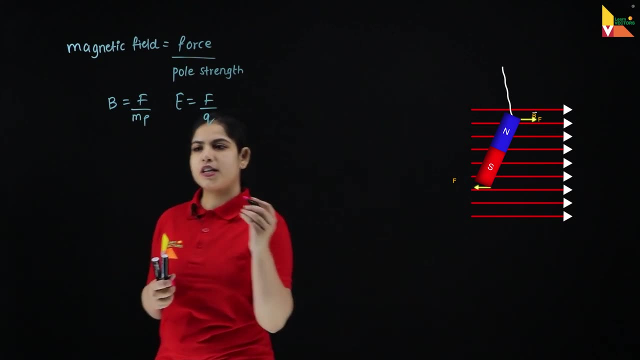 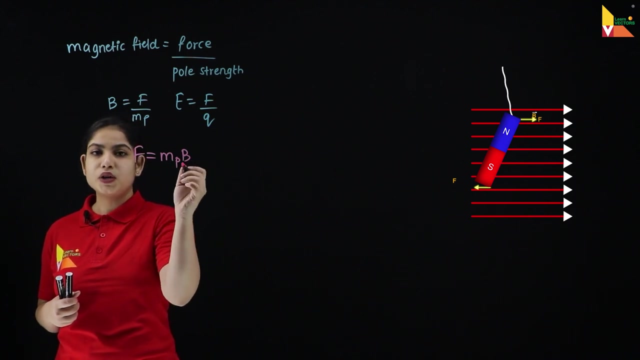 of this torque. there is a force also experienced right. so the force experienced by the North Pole is in the direction of the magnetic field and this force is what this force is. F is equals to MP into B. again, MP is what it is: the pole strength. B is the magnetic field and F is what F is the 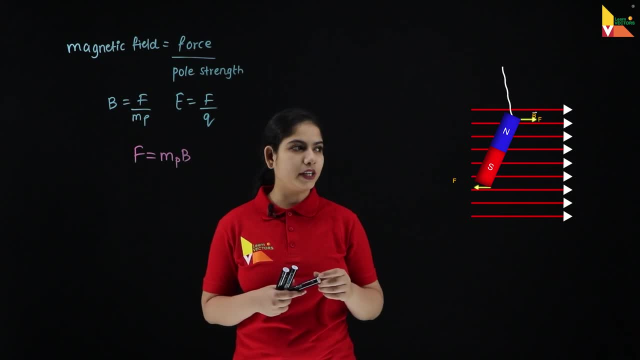 force that is experienced by the North Pole. okay, so if the direction of North Pole is along the magnetic field, then what will be the direction of South Pole, opposite to the direction of North Pole, right, and whenever such cases appear, at that time, what is generated? this is nothing but an 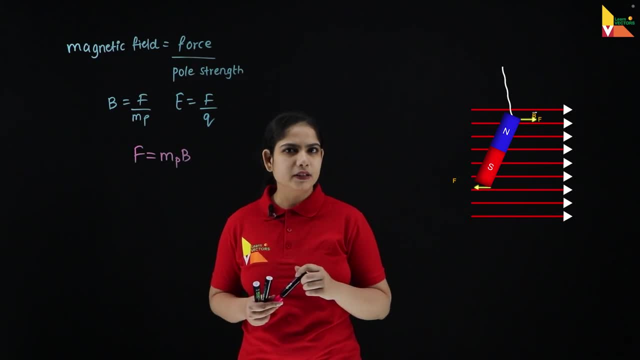 example of a couple right and in couple, the rotational motion comes into picture right and that this bar magnet is experiencing torque. okay, whenever there is opposite forces, at that time what do we observe? that there is a rotational motion over here. if I am applying the force in, 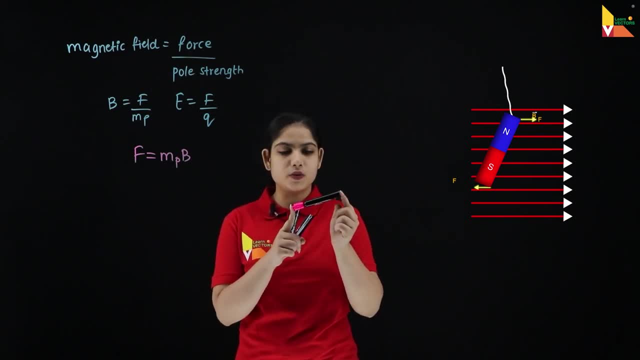 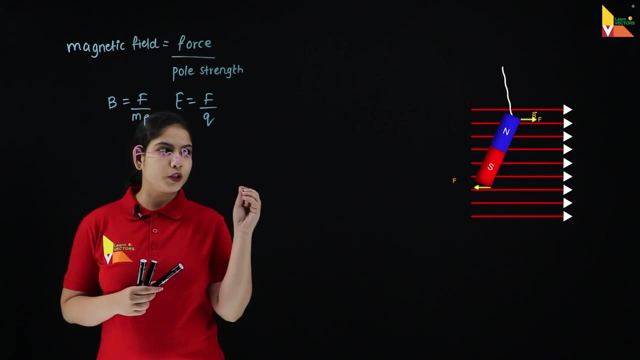 the downward direction and this force in the upward direction. this pen is what this pen is rotating now, right. so this is nothing but what. this is an example of a couple. so over here, torque is acting on that bar magnet, right? oh, what is the basic formula for torque that we have studied in? 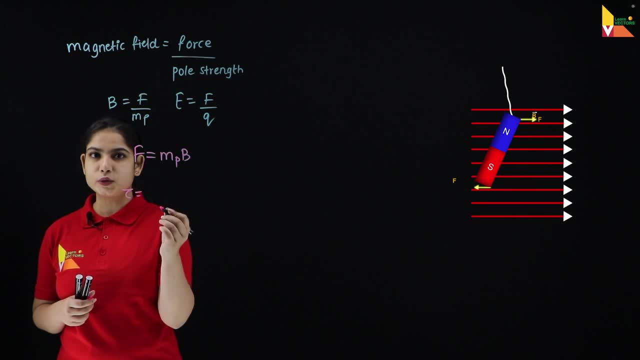 our lower classes. torque is given by force into the perpendicular distance right. force into distance. this is the formula for torque. so, over here, what is force? we have the value for force. force is mp into b right. and now what is the perpendicular distance over here? let us again go back to the 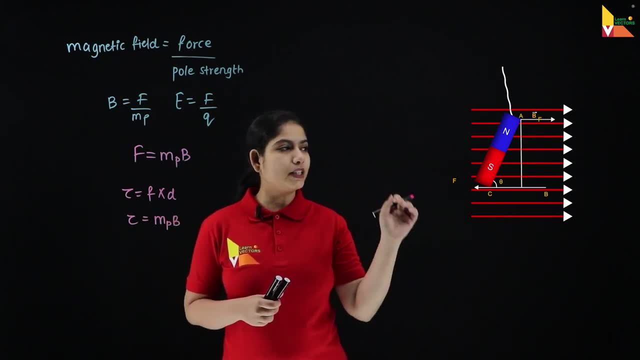 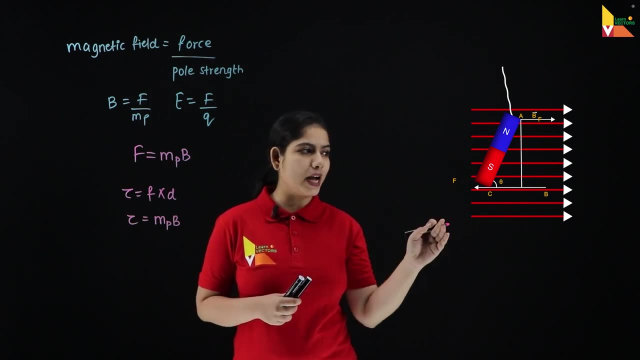 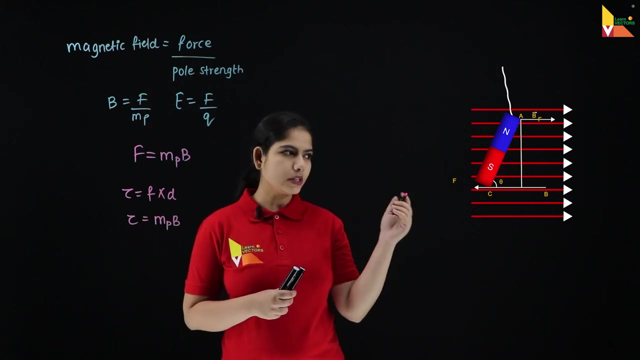 figure you over here. let us extend these two forces: the force that is acting on the North Pole and the force that is acting on the South Pole. let us extend these two lines and what do we observe? that there is a formation of triangle over there, right, and the angle of deflection is given by what? 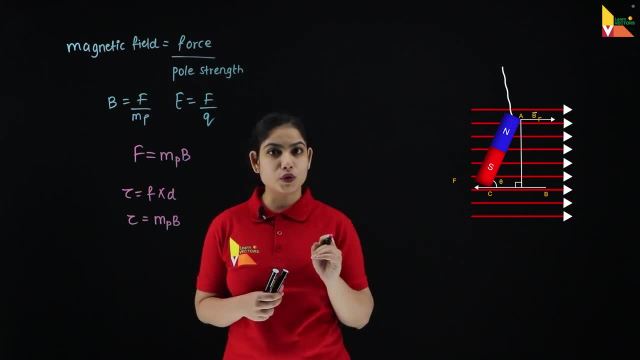 theta and a right angle is also formed. so over here, by looking at this picture, what can we apply over here? the rules for trickery, so the rules for trigonometry? we need to find out the perpendicular distance, and the perpendicular distance in this case is what? the distance from a to b, right the side, a, b is the. 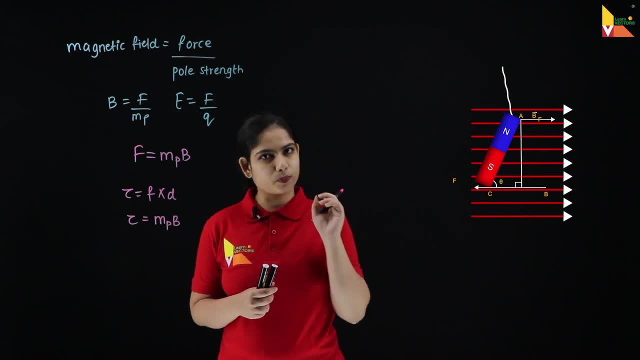 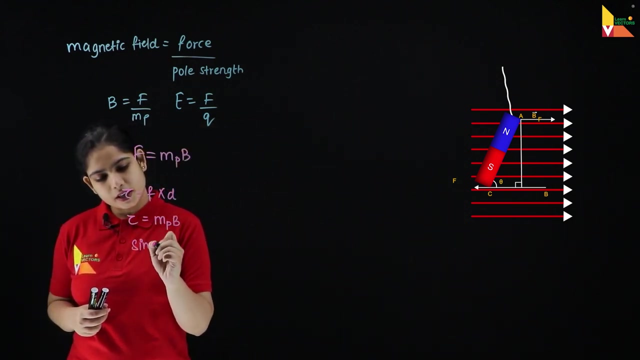 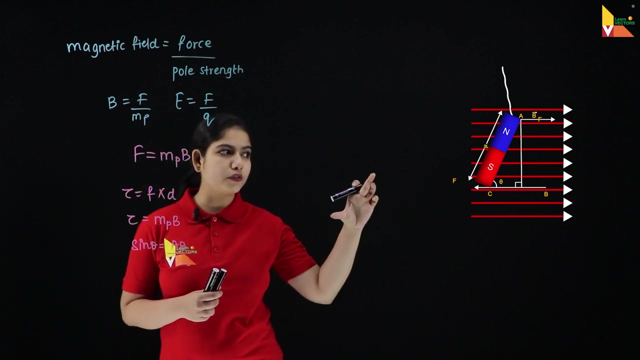 perpendicular distance. so we need to find out the value of a, b over here what we are going to use. we are going to use sine theta because sine theta is opposite upon Hypotenus. what is the opposite side. a, b theta is equals to AB upon 2L. 2L is what? 2L is the length of the bar magnet right. 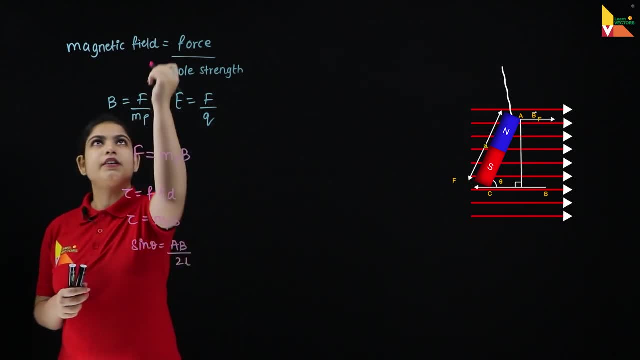 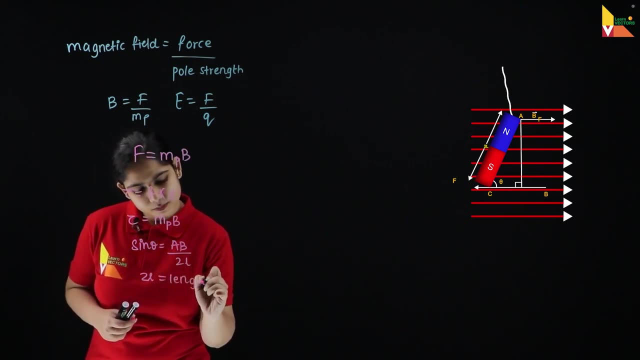 2L is the total length of the bar magnet. Let us write it over here: 2L is what? 2L is the length of bar magnet. okay, And what do we have to find out? We have to find out. 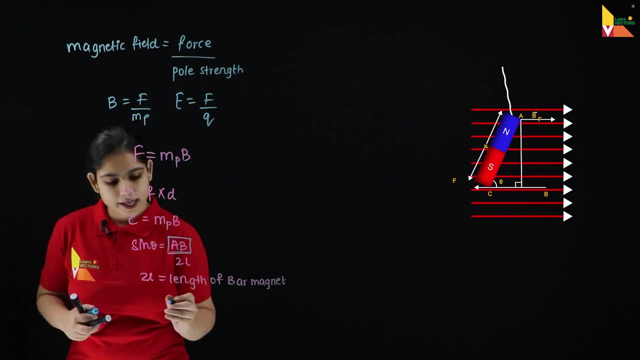 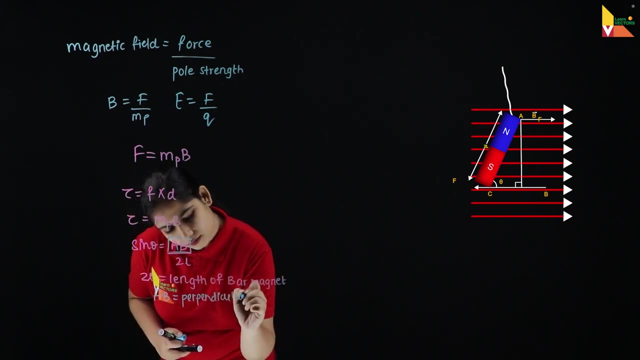 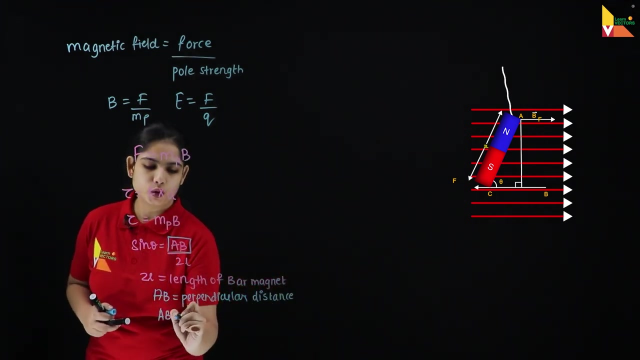 the value for AB, because AB is what AB is: the perpendicular distance. So what will be AB? AB is 2L sin theta, And this is nothing but what. This is the distance. So now we will substitute this, We will substitute this value in the above equation for torque, and then what we will? 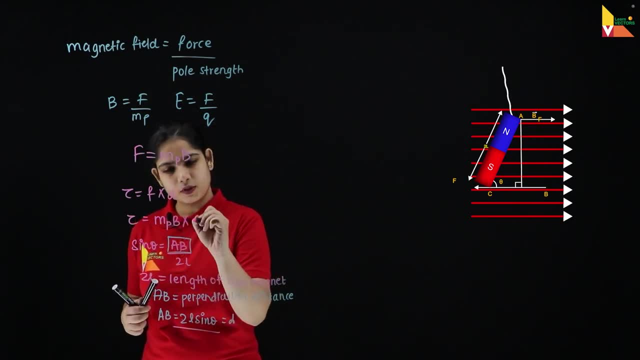 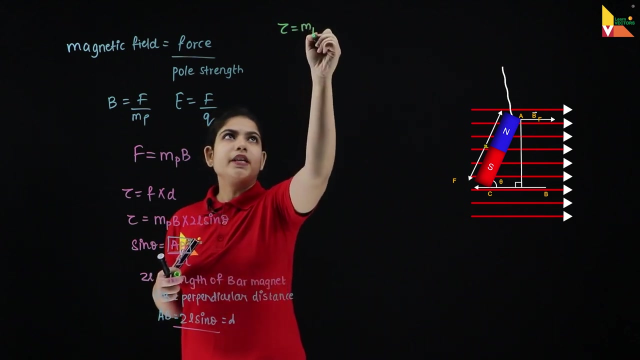 get MP into B is 2L sin theta. right, Understood how we are going to write this. So we have this equation with us for torque, which is MP into B, into 2L sin theta. Now this term and this value are equal to 2L sin theta. So we have this equation with us for torque. 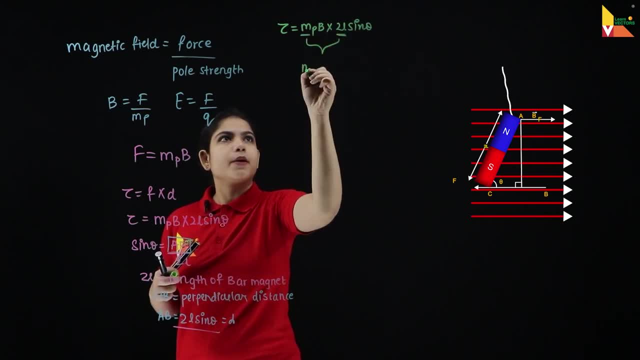 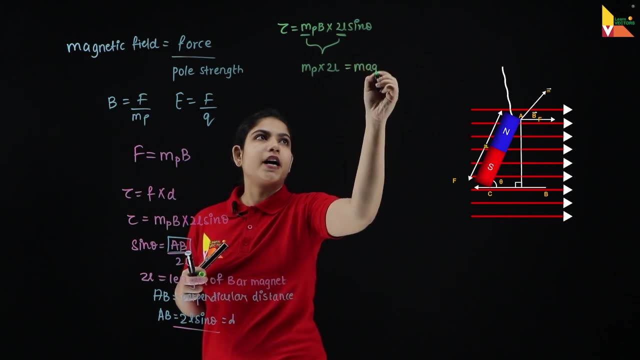 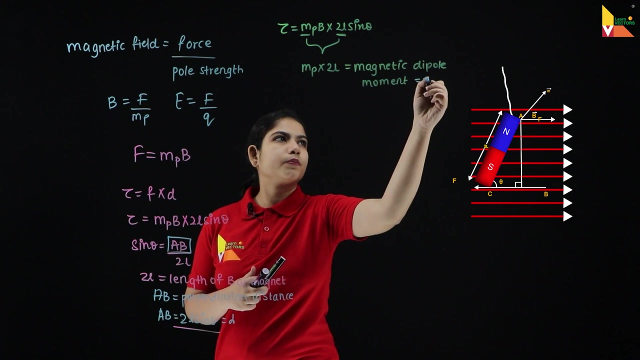 and this value are equal to 2L sin theta. Now, this is what MP into 2L. This is what This term is called as magnetic dipole moment: magnetic dipole moment which is denoted by M, small m. okay, So we are going to substitute these two terms. So we are going to substitute. 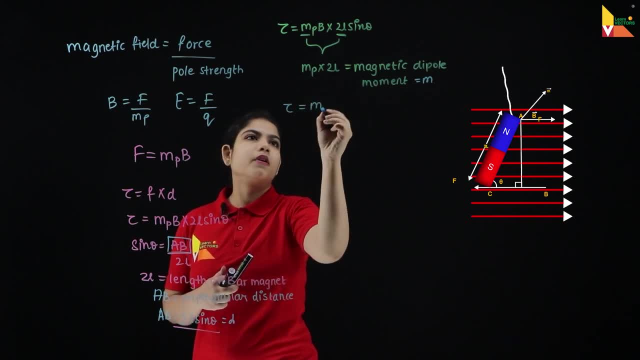 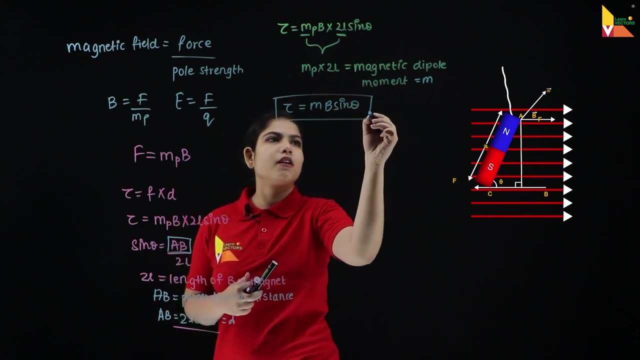 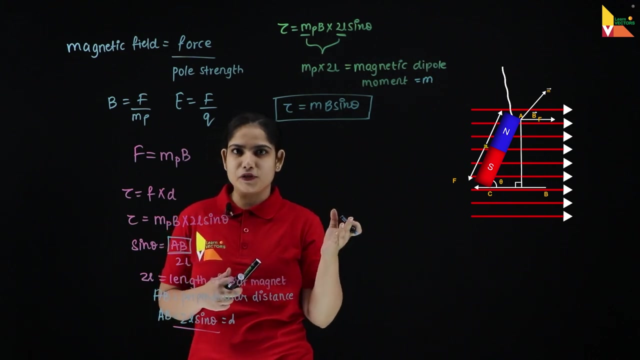 these two terms as M, B, sine theta, and this is the equation which is given to us in the textbook, right, what is M over here? M is the magnetic dipole, moment B is the magnetic field and sine theta is sine theta, right? and if we want to write this, 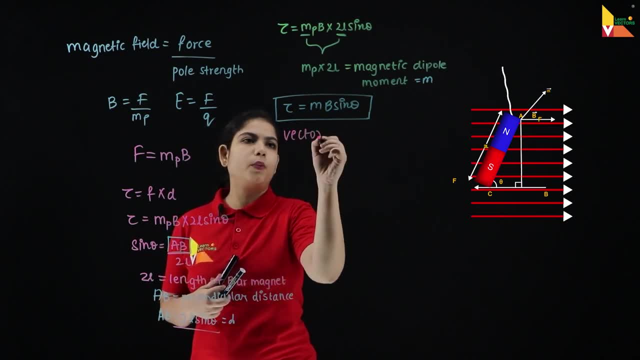 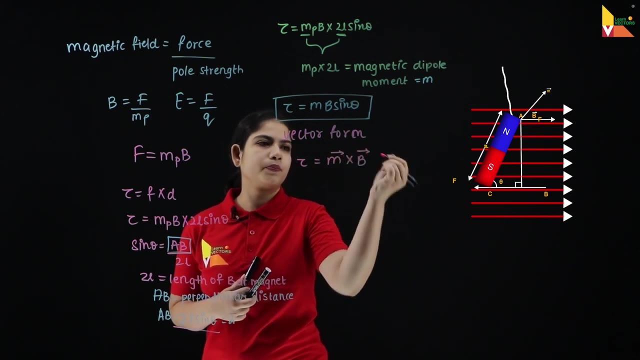 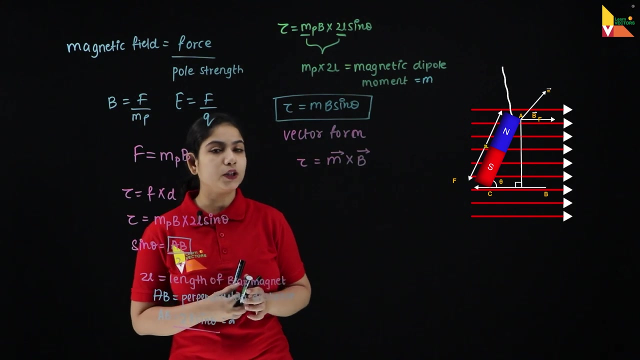 in the vector form. in the vector form, this equation will be? what vector form? what will be the equation? tau is equals to M cross B. now the direction of M vector and B vector is given over here. okay, so according to the right-hand rule, if we want to check the direction of torque,